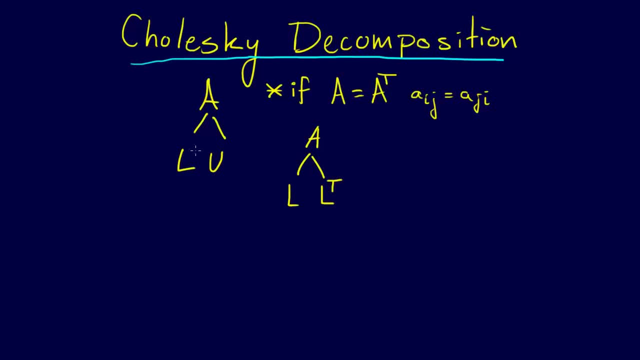 Now this is really cool because it's actually a special case of this L and U, because L is this lower triangular matrix and U is the upper triangular matrix. Well, the transpose of L is an upper triangular matrix And so if that U is actually equal to L transpose, then we have a Cholesky decomposition and we can do the Cholesky decomposition and these actually, it turns out, are a really great tool. 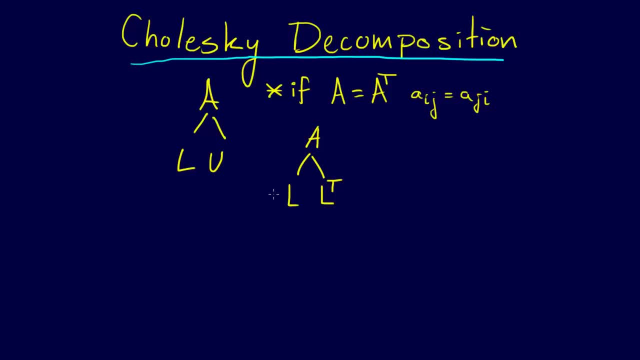 They can save computation time as well as storage space, And so this is a good thing. as we talked about So in Cholesky decomposition, then what we do is we just say: then A equals L, L transpose, and then we can write out the equations for that right. 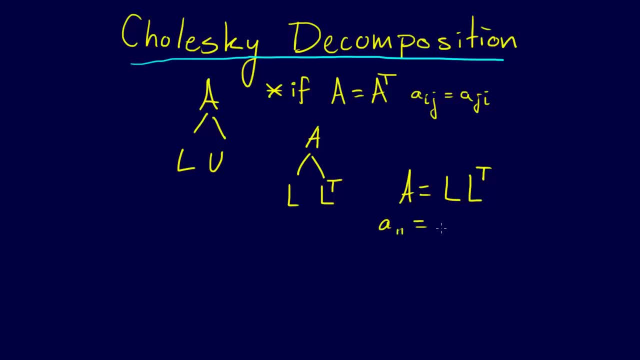 A11 equals L. it would be L11 squared, I believe, right? Yeah, yeah, I'm pretty sure. Yeah, so we can write out. we just keep writing out all the other terms there and what we get is a whole bunch of equations. but we can write those equations in summation notation, which is what they've done in the book. 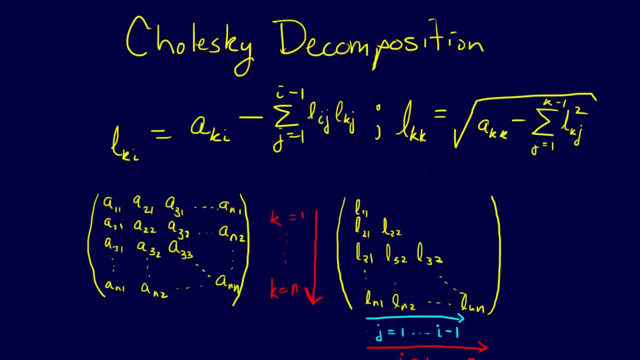 And I just Let me move down here. I just copied down those equations so that it was easier, saved some writing time here. So we have LKI. the KI element is equal to AKI minus. the sum from J equals 1 to I minus 1 of LIJ, LKJ. 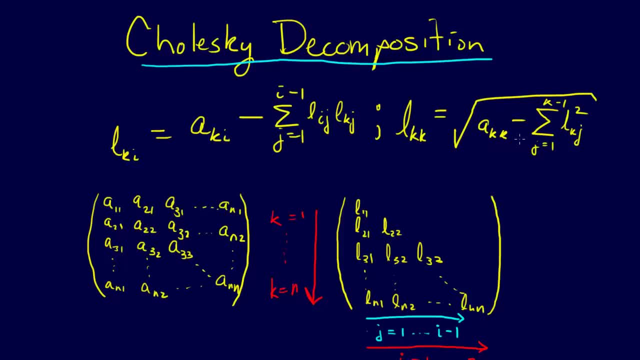 And then we have a second equation: LKK equals the square root of AKK minus the sum from J equals 1 to K minus 1 of LKJ squared. Now, if that makes any sense to you, well, that's great. 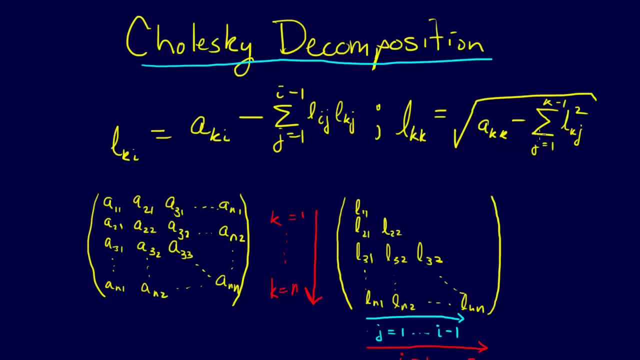 You're faster than I am. But what we have to do here so we can really understand what's going on, is: let's take a look at these. Let's take a look at how we move through in these equations. So the first index we can look at 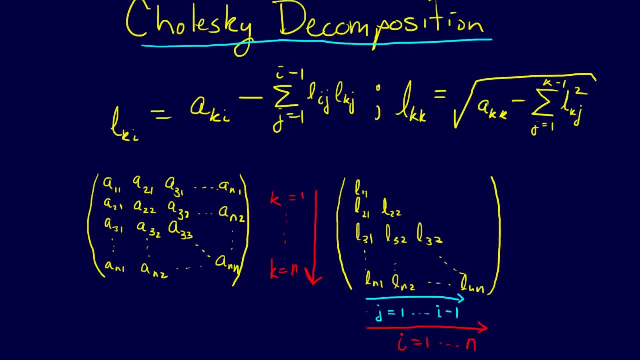 And then let me move down here so we can see this other index as well. The first index we're going to look at That is K. okay, K is our main index. You can see it shows up here and it shows up here. 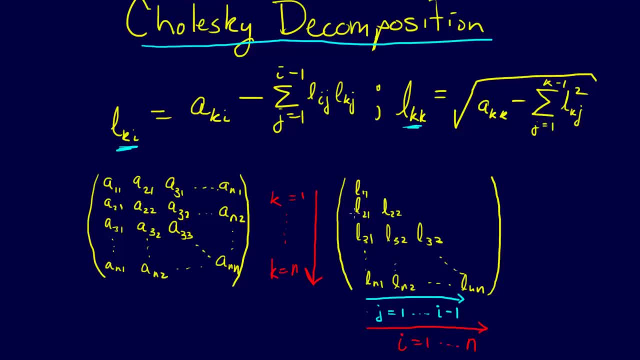 We've got this LKK and LKI And so K is our main index And K moves from 1 to N. K is like our outer loop. okay, So we move from 1 to N. So we're going to start on row 1 and we're. 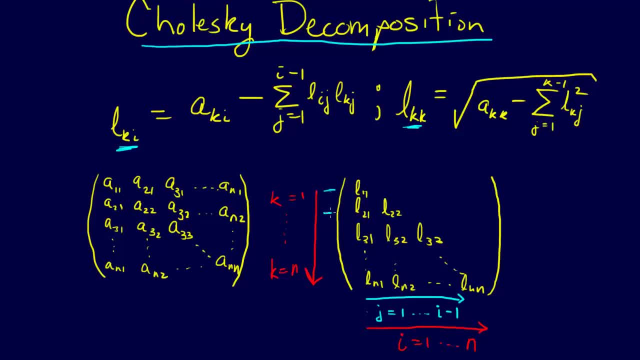 So we're going to: First we'll do the L11 element, Then we're going to start On row 2 and we'll do these elements. We start, Then we go to row 3 and we do these, Then we go to row 4.. 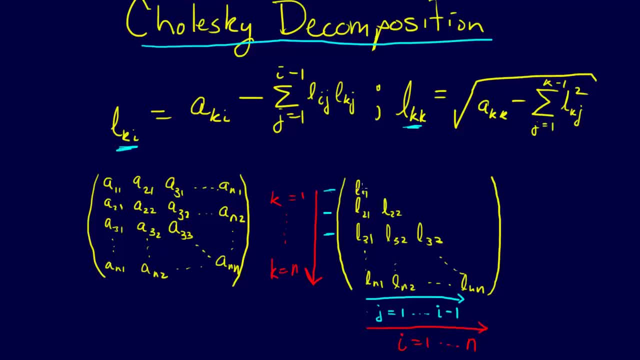 So this is how this L matrix is populated as we go through, First here and then here and then here. But in order to see that, you need to look at the other index. The other index is I, And I starts from 1 and goes to N. 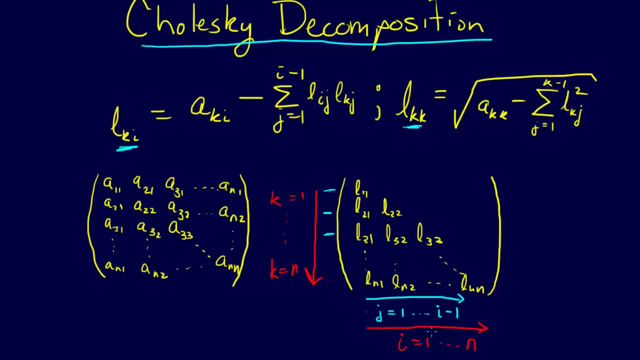 But, But, But, But, But. this particular age is 1.. It starts at 1. And goes to what ever the current Current element is. So maybe, Maybe I shouldn't have written N there. So whatever you're currently on, 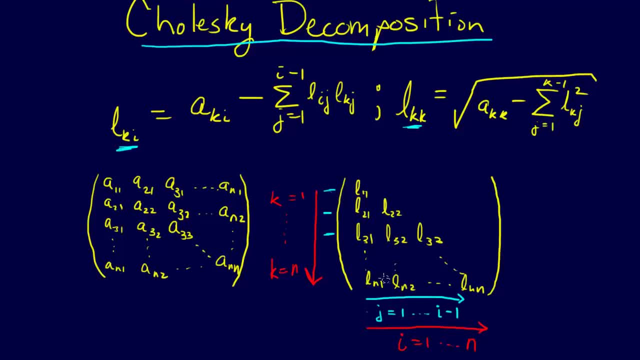 Well, it is going to go to N. Okay, so we, In other words, what that means putting all that together then- is: this is the first element that gets populated. Then the second element that gets populated is this one. this is the third. then we move down here. this is the fourth, this is the fifth, this is the sixth, seventh, eighth, ninth, so far and so forth, and this will be then, and then we're going to move across here. let's see if this is the- I don't know what number it'll be down to by the time we get here in general, but anyway it'll go: this one, then this one, and then we'll populate. 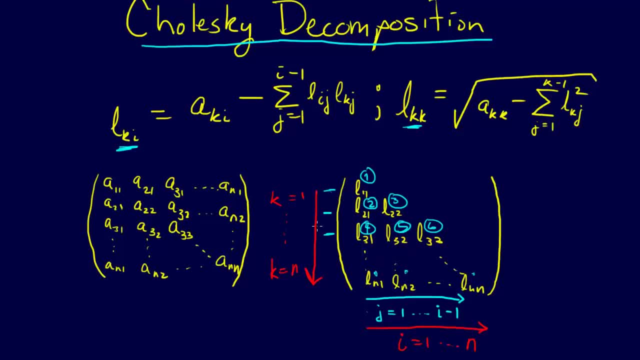 This one in the very last. okay, so this is how we move through with our indices K and I. Now we have to look at this index J. alright, so first, when we move through here, the first, and at any step when we're computing an element, at any step, we're only going to use one of these two equations, not both of them at the same time, and so we use this first equation when K is not equal to I. 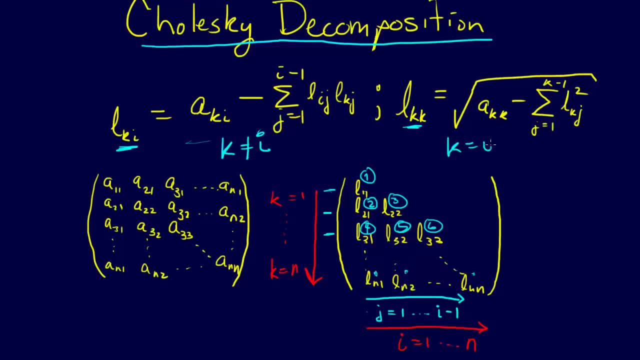 and we use this second equation when K equals I, or that's why they just use KK. so that's it. and then this second index, J. so J goes from 1 to I minus 1, or from 1 to K minus 1, and K minus 1 is really I minus 1 when K equals I. so you can really think of it as doing the same thing. 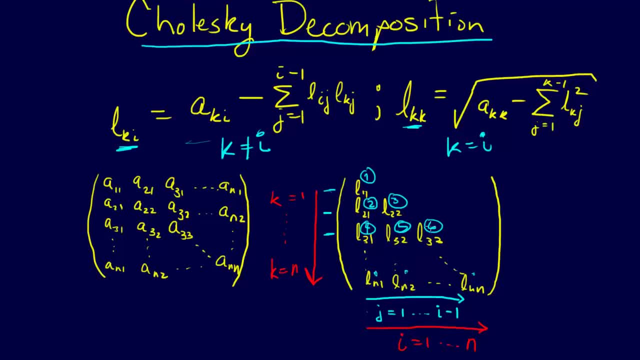 and so what that means is, if we're working, for example, on this element right here, that's going to be the sixth one that gets done. we're going to be summing elements starting here, right starting here, and moving over here here and so forth. 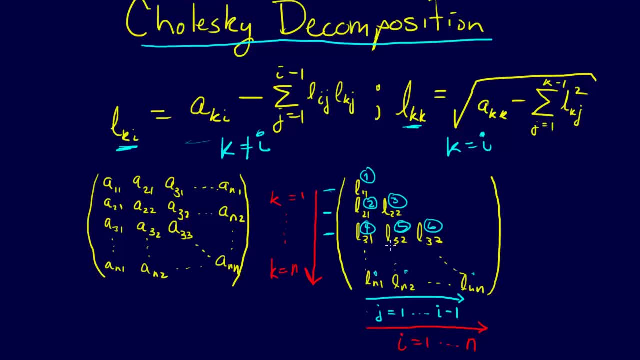 so that's the idea behind what's going on there. Same here. we're going to be using these elements to compute this entry. alright, now you'll see that a little more in the example. we'll run through real quick in the next video. 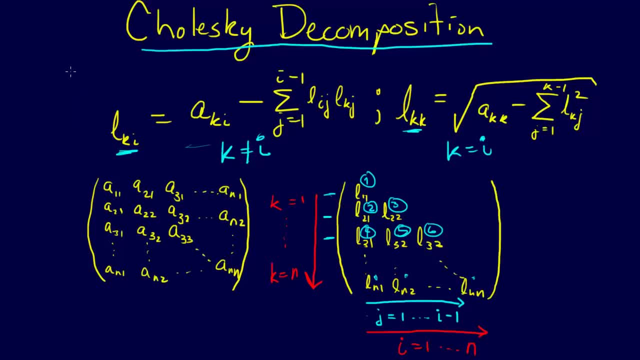 There is actually one other comment that I wanted to make before we move on. If you remember, we have this decomposition: A equals L, L transpose. this is about as close as we can get to taking the square root of a matrix, and it's actually for that reason that you see, in this part of the equation, this square root appear here, because we're essentially taking the square root- L- L transpose, we're multiplying two matrices that are 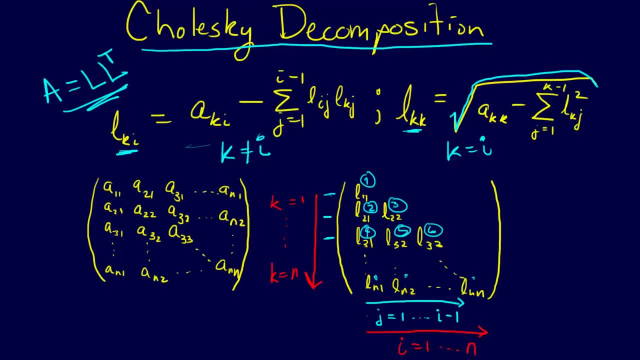 you know we're multiplying two matrices that are. you know we're multiplying two matrices that are basically the same matrix together to get A.